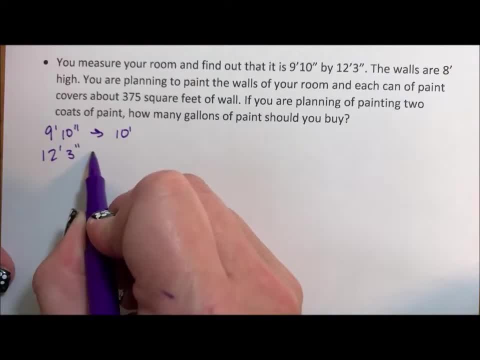 And I would take the 12 feet 3 inches and probably just make that 12 feet so that I have a room that's 10 feet by 12 feet- Feet, not inches. And then you know we have 8 feet high because we have to make it 3D. 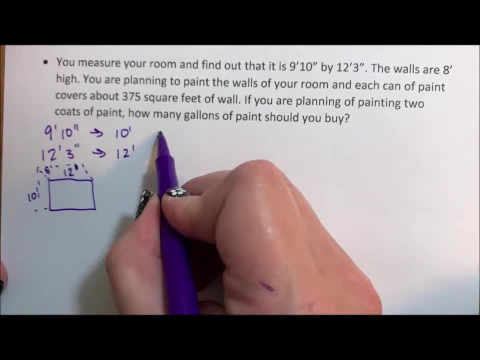 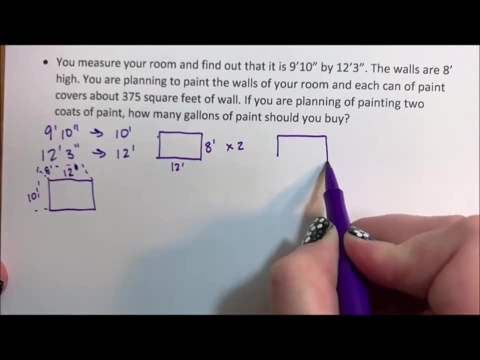 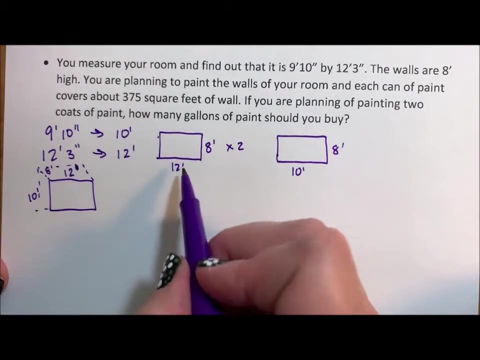 So each wall? we have two walls that are 12 feet by 8 feet. We have two walls that are 10 feet by 8 feet that we need to paint, So 12 by 8. I have to multiply those, So 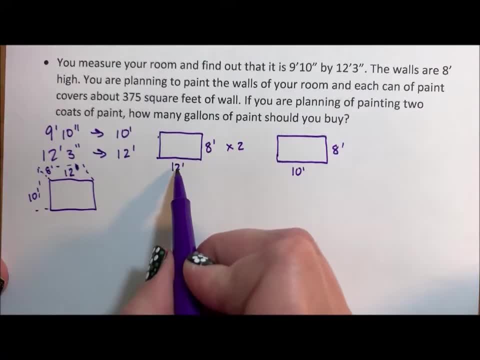 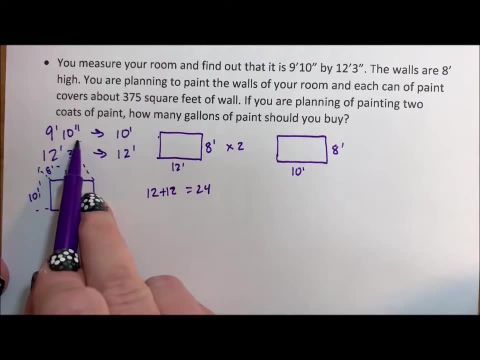 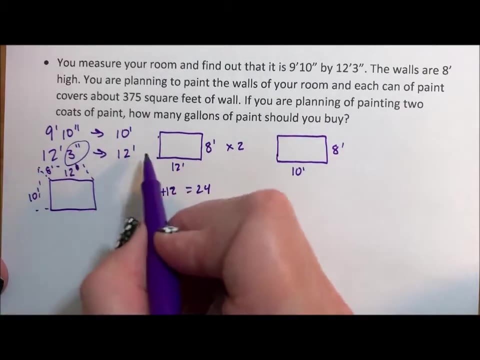 I'm starting to look at this: 12 plus 12 is 24.. And it's a little bit short, right? I'd rather buy too much paint than not enough paint. So this is how we estimate. How do we make this simple? If I made this: 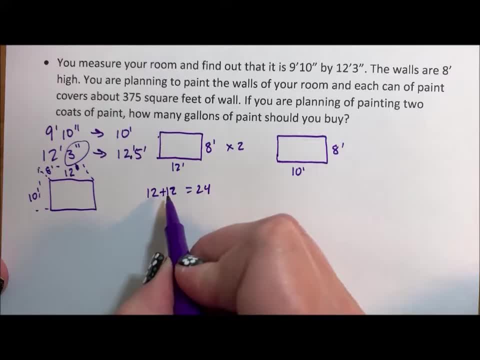 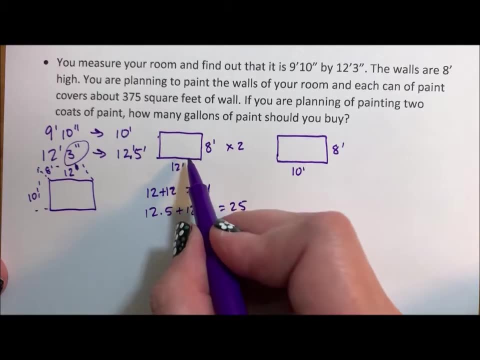 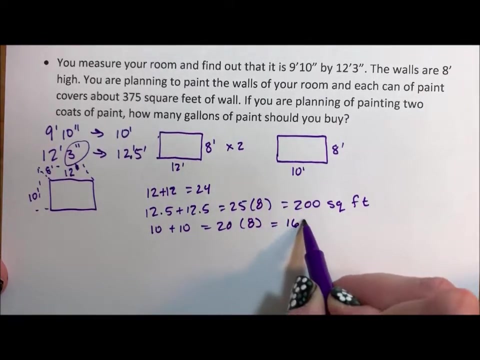 12 and a half feet instead of 12,. well, 12 and a half plus 12 and a half is 25.. 25 for the two walls times 8 is 200 square feet. 10 is easy. 10 plus 10 is 20.. And 20 times 8 is 160. And if we add those together we have 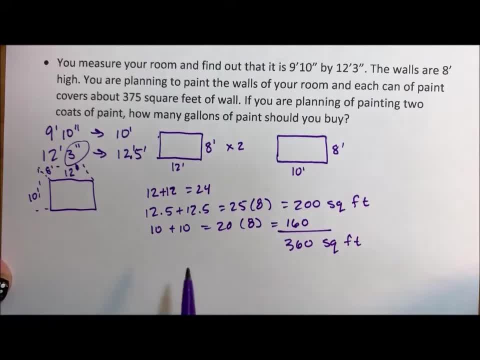 360 square feet. So what I did was I took the 12.3, made it 12 and a half, 12 and a half each of the two. 12 and a half plus 12 and a half is 25.. 25 times 8 is 200.. 10 plus 10. 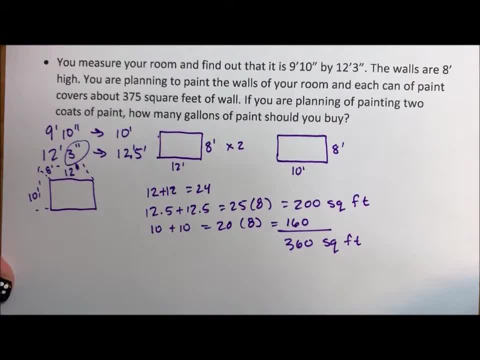 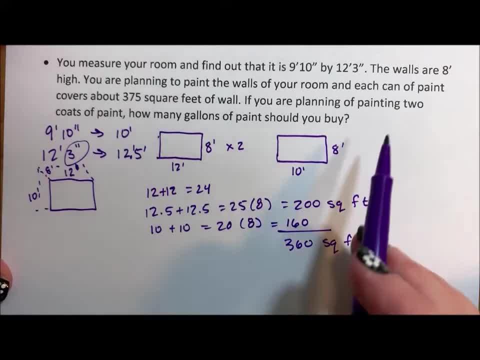 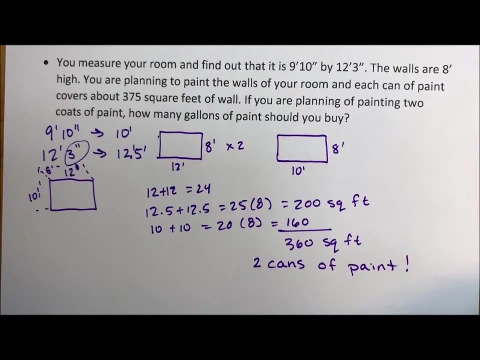 paint can should cover all of my walls, but I want to do two coats, So I should get two cans of paint. So in there you saw how estimation happens and how you can alter your estimation to work for you. 12. So I started estimating up and estimating down, but then I realized my estimation would